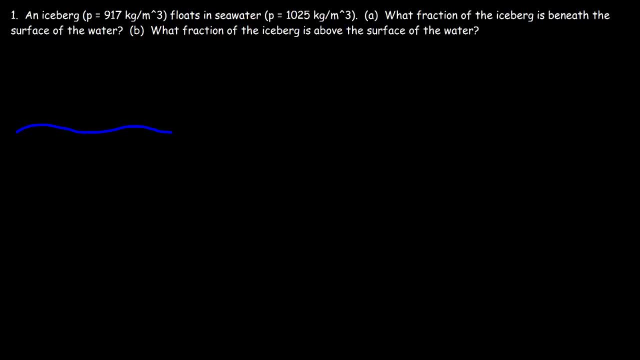 So, as always, let's draw a picture. So let's say: this is the sea And we know that ice floats on seawater, because ice is less dense than seawater. So we need to calculate the fraction that is submerged, that is, the fraction of the ice cube or iceberg beneath the seawater and the portion that is above the seawater. 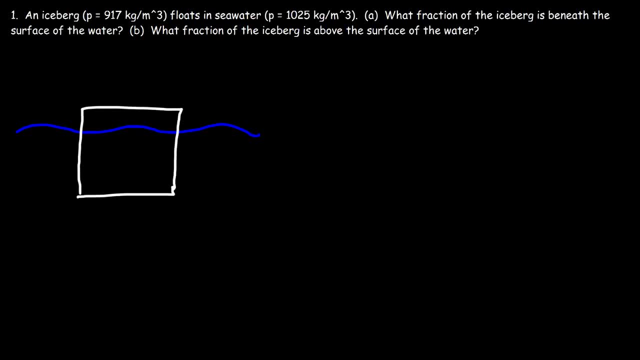 So how can we do it? Well, first let's create a free body diagram. Now, if the ice is floating, that means that it's stationary, It's not going up, it's not going down, it's staying where it is. 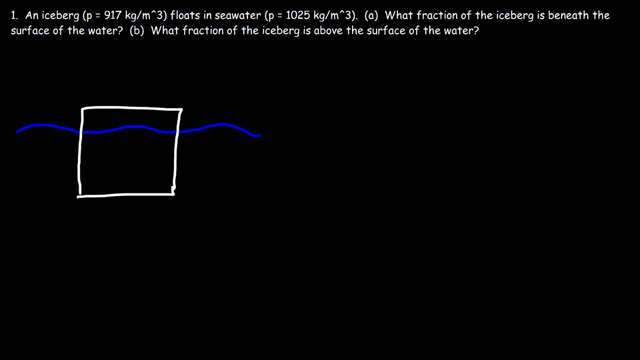 So the net force in the y direction has to be zero. So the buoyant force which pushes the block up has to be equal to the weight force, such that the net force in the y direction is zero. So we can set those two equal to each other. 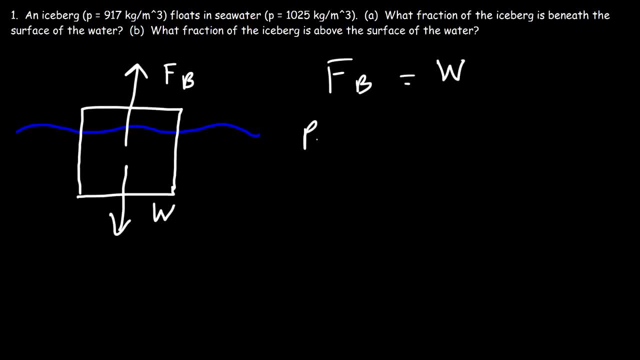 Now, the buoyant force is the product of the density of the fluid times, the volume submerged, so that is the volume of the iceberg that is beneath the water. so that's Vs multiplied by the gravitational acceleration, And the weight of the object is simply mg. 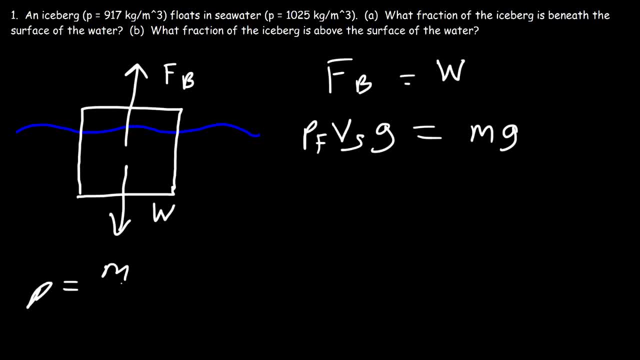 Now, density is mass divided by volume. So if we multiply both sides by the volume, mass is density times volume. So let's replace m with that. So the mass of the object is the density of the object multiplied by the entire volume of the object times g. 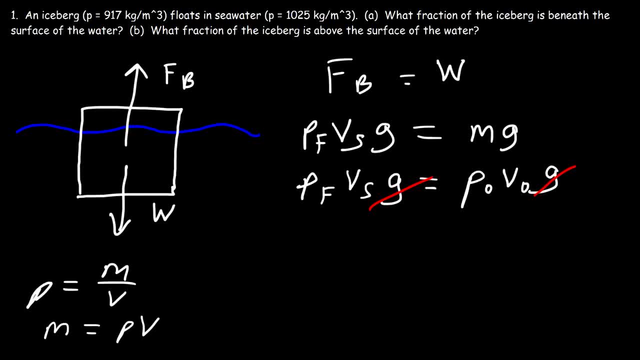 And so we could cancel g. So this is the relation that we need. The density of the fluid times the volume of the object that is submerged is equal to the density of the object times the volume of the object. Now I'm going to draw some pictures so you can clearly see what Vs and Vo represent. 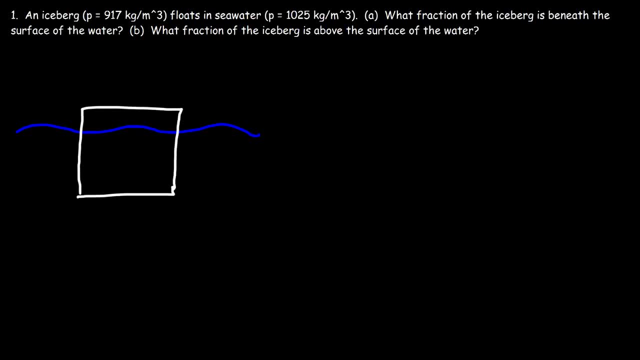 So how can we do it? Well, first let's create a free body diagram. Now, if the ice is floating, that means that it's stationary, It's not going up, it's not going down, it's staying where it is. 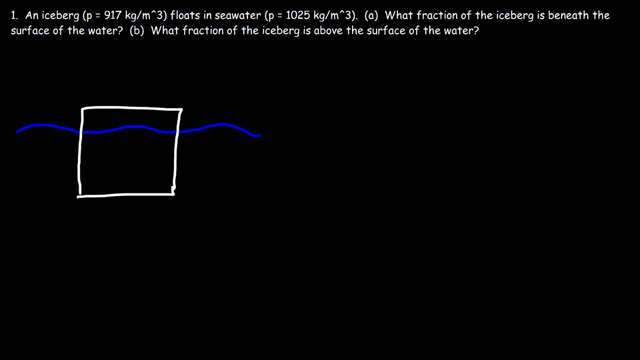 So the net force in the y direction has to be zero. So the buoyant force which pushes the block up has to be equal to the weight force, such that the net force in the y direction is zero. So we can set those two equal to each other. 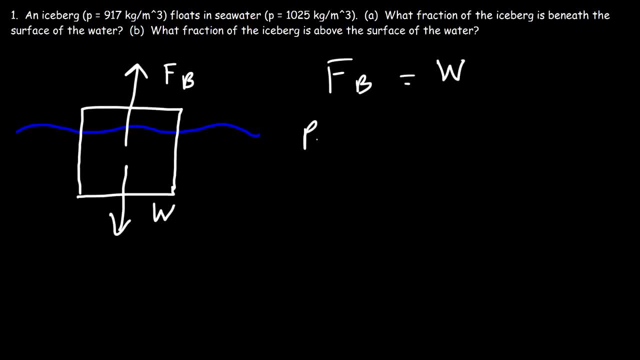 Now, the buoyant force is the product of the density of the fluid times, the volume submerged, so that is the volume of the iceberg that is beneath the water. so that's Vs multiplied by the gravitational acceleration, And the weight of the object is simply mg. 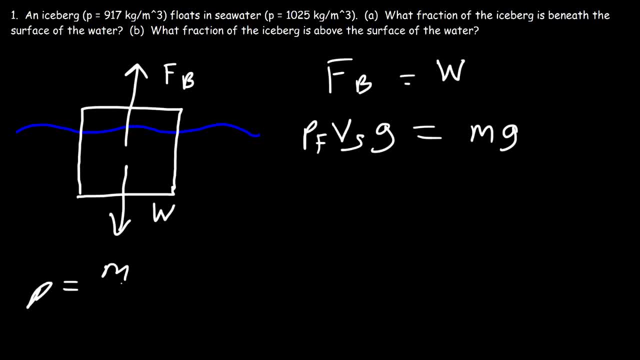 Now, density is mass divided by volume. So if we multiply both sides by the volume, mass is density times volume. So let's replace m with that. So the mass of the object is the density of the object multiplied by the entire volume of the object times g. 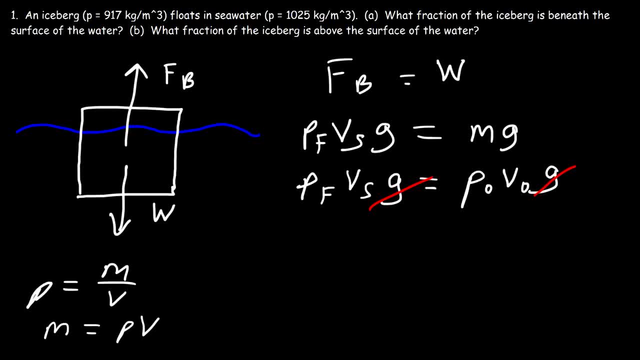 And so we could cancel g. So this is the relation that we need. The density of the fluid times the volume of the object that is submerged is equal to the density of the object times the volume of the object. Now I'm going to draw some pictures so you can clearly see what Vs and Vo represent. 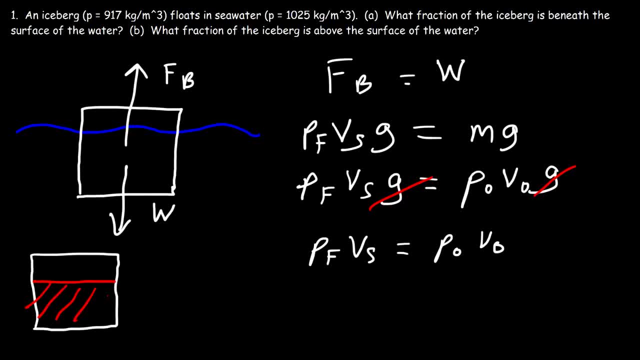 So Vs is the portion that is submerged, that is, the portion that is in the fluid. So that's Vs. Vo represents the entire volume of the object. Make sure you understand that. So now we can answer this question In order to find the fraction of the iceberg that is beneath the surface of the water. 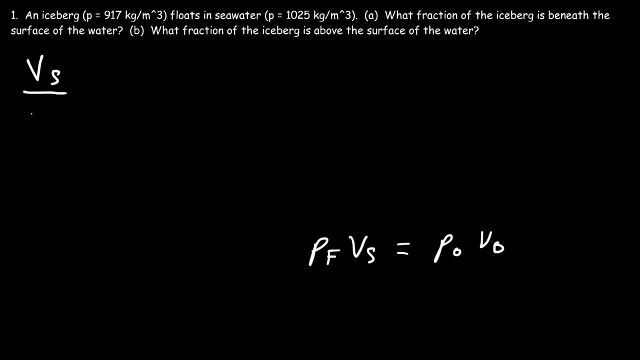 we need to take the volume that is submerged and divide it by the total volume of the iceberg. So in this case we need to divide both sides by Vo and at the same time let's divide both sides by Pf. So on the right side those will cancel. 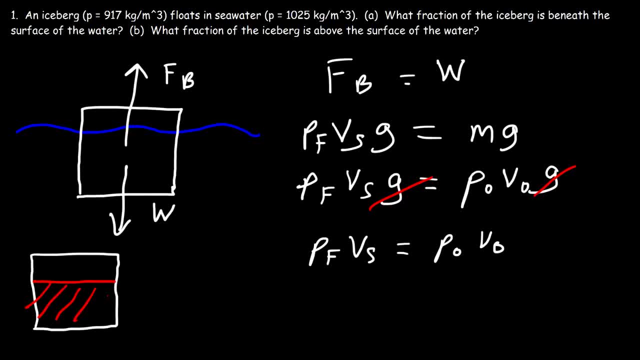 So Vs is the portion that is submerged, that is, the portion that is in the fluid. So that's Vs. Vo represents the entire volume of the object. Make sure you understand that. So now we can answer this question In order to find the fraction of the iceberg that is beneath the surface of the water. 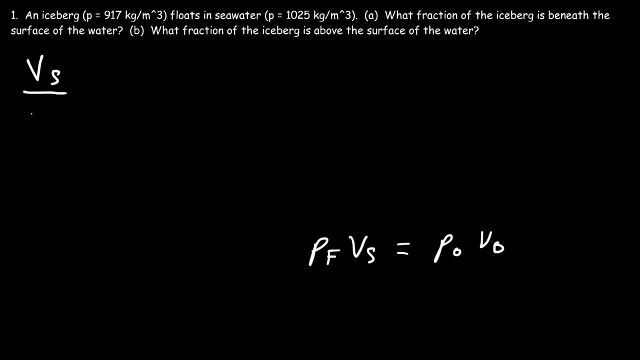 we need to take the volume that is submerged and divide it by the total volume of the iceberg. So in this case we need to divide both sides by Vo and at the same time let's divide both sides by Pf. So on the right side those will cancel. 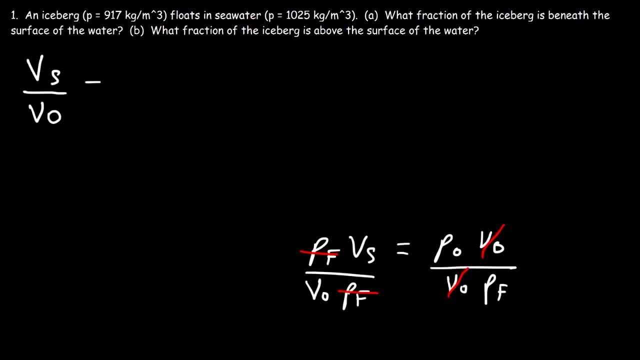 On the left side. these two will cancel. So the volume submerged divided by the volume of the object, that's equal to the density of the object divided by the density of the fluid. And so the density of the iceberg is 917 kilograms per cubic meter. 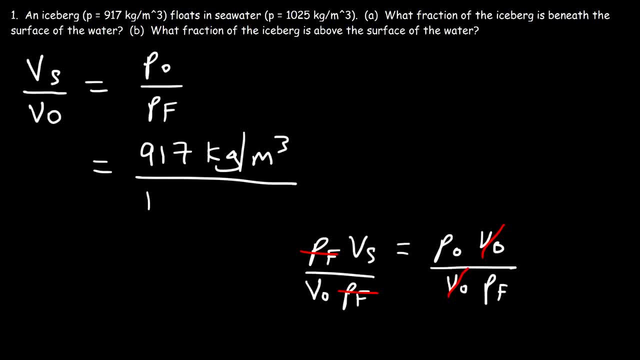 And the density of the fluid which is seawater, that's 1025.. So this is going to give us a unitless fraction. So the fraction of the iceberg that is beneath the surface of water is 0.895.. And the fraction that is above the surface of water is 1 minus that number. 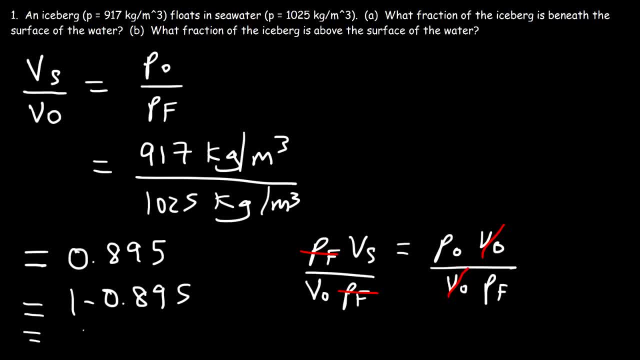 Which is 0.105.. So what does this mean in terms of practical stuff? So what this means is that in seawater, which is different from pure water, 89.5% of the iceberg is beneath the seawater. And let's say, if you're on a boat, 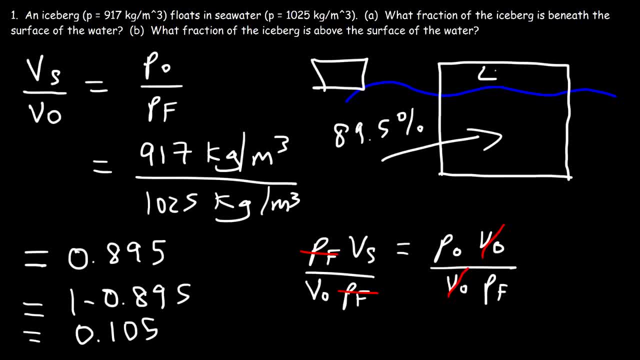 Let's say, if you're on a boat. Let's say: if you're on a boat, What you see is only a fraction of the iceberg on top of the seawater. So you're only looking at 10.5% of the iceberg. 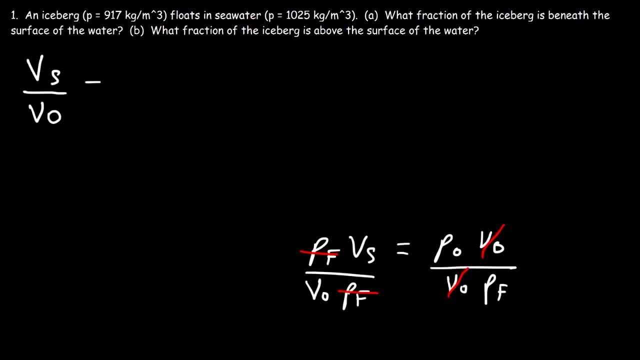 On the left side. these two will cancel. So the volume submerged divided by the volume of the object, that's equal to the density of the object divided by the density of the fluid. And so the density of the iceberg is 917 kilograms per cubic meter. 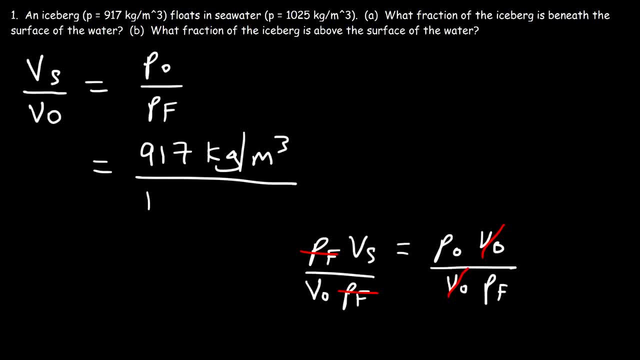 And the density of the fluid which is seawater, that's 1025.. So this is going to give us a unitless fraction. So the fraction of the iceberg that is beneath the surface of water is 0.895.. And the fraction that is above the surface of water is 1 minus that number. 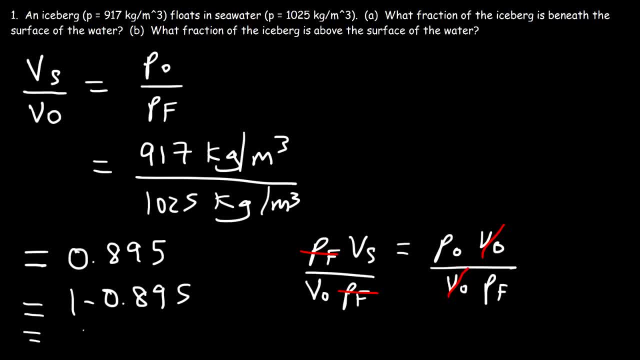 Which is 0.105.. So what does this mean in terms of practical stuff? So what this means is that in seawater, which is different from pure water, 89.5% of the iceberg is beneath the seawater. And let's say, if you're on a boat, 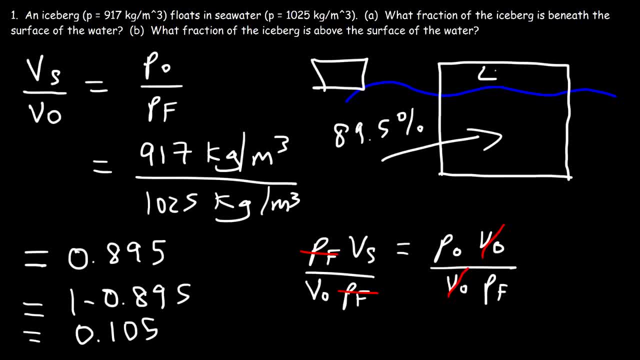 Let's say, if you're on a boat. Let's say: if you're on a boat, What you see is only a fraction of the iceberg on top of the seawater. So you're only looking at 10.5% of the iceberg. 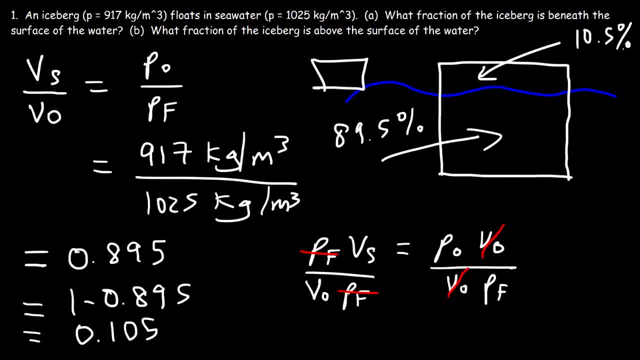 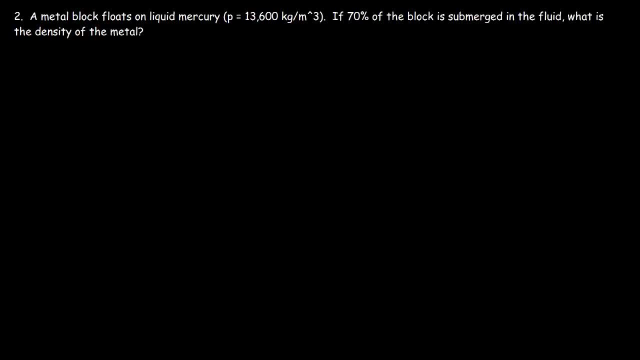 The other 90% is beneath the seawater. Number two: A metal block floats on liquid mercury. If 70% of the block is submerged in the fluid, what is the density of the metal? So let's draw a picture. So let's say that we're on a boat. 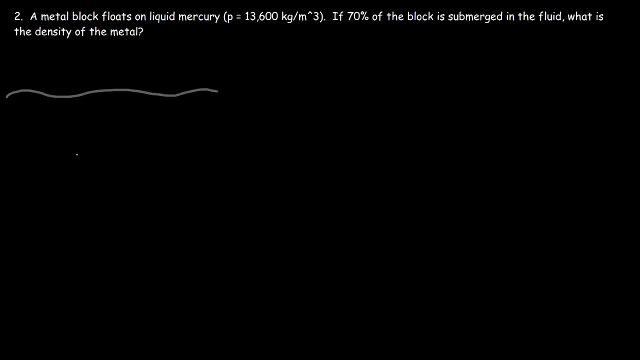 Let's say this is liquid mercury And this is the metal block. So 70% is submerged. So we could pick a number. Let's say the total volume is 10 cubic meters. It really doesn't matter, It's the ratio, that's what's important. 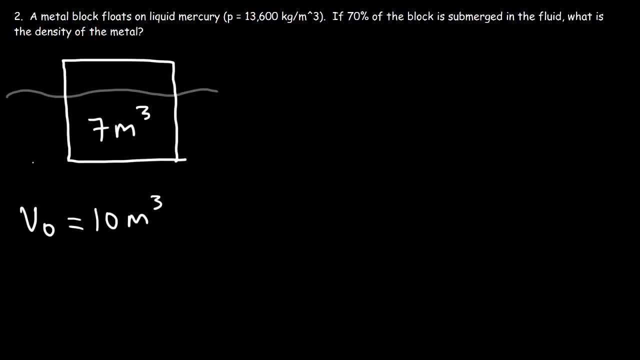 That means 7 cubic meters has to be beneath the fluid, The other 3 has to be above it. 7 over 10 is 70%. So now let's calculate the density of the metal. So the density of the fluid times the volume submerged is equal to the density of the object times the volume of the object. 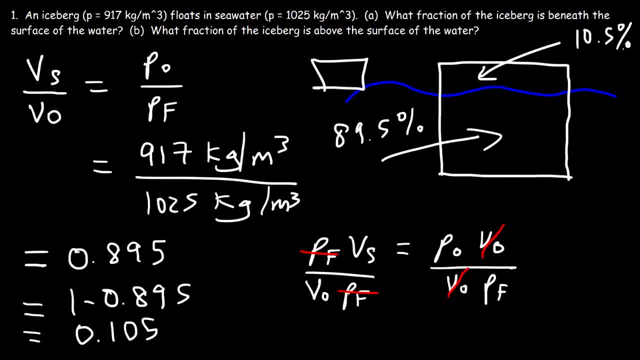 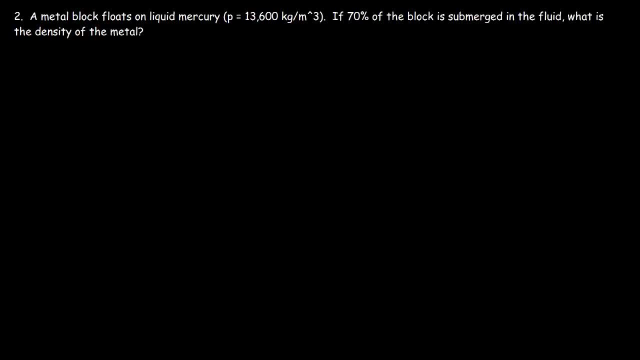 The other 90% is beneath the seawater. Number two: A metal block floats on liquid mercury. If 70% of the block is submerged in the fluid, what is the density of the metal? So let's draw a picture. So let's say that we're on a boat. 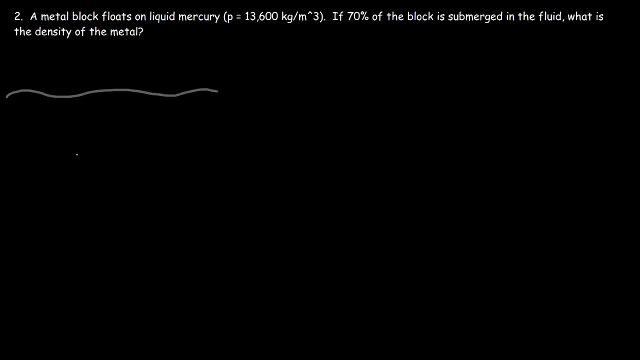 Let's say this is liquid mercury And this is the metal block. So 70% is submerged. So we could pick a number. Let's say the total volume is 10 cubic meters. It really doesn't matter, It's the ratio, that's what's important. 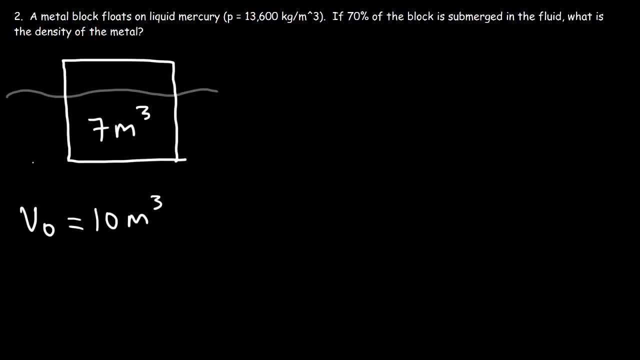 That means 7 cubic meters has to be beneath the fluid, The other 3 has to be above it. 7 over 10 is 70%. So now let's calculate the density of the metal. So the density of the fluid times the volume submerged is equal to the density of the object times the volume of the object. 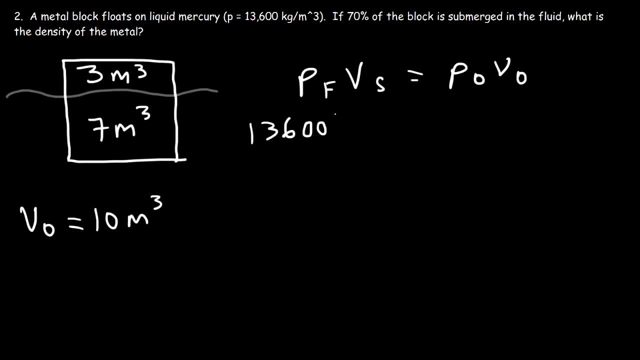 So we have the density of the fluid, That's liquid mercury, That's 13,600.. The volume submerged is 7.. And we're looking for the density of the metal, That is, the metal block And the volume of the entire object. 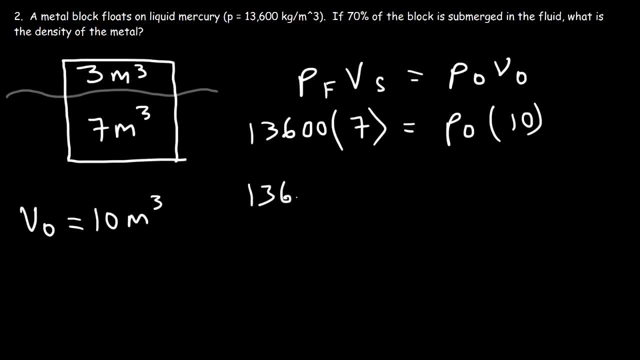 And the volume of the entire object is 10.. So it's going to be 13,600 times 7 over 10.. So if you need to find the density of the object, it's the density of the fluid times, the volume submerged divided by the volume of the object. 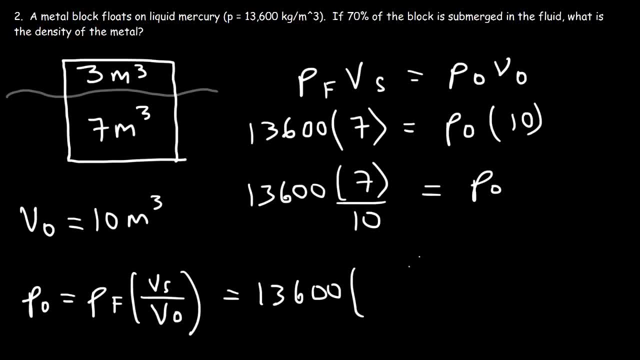 So that's 13,600 times 7 over 10,, which is 0.7 or 70%. So therefore, the density of the metal is simply 70% of the volume of the object, And that's the density of the density of mercury. 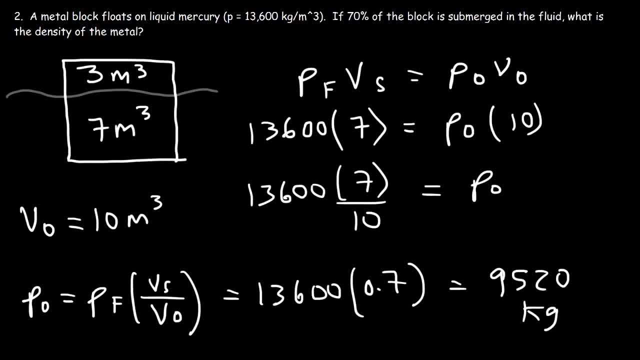 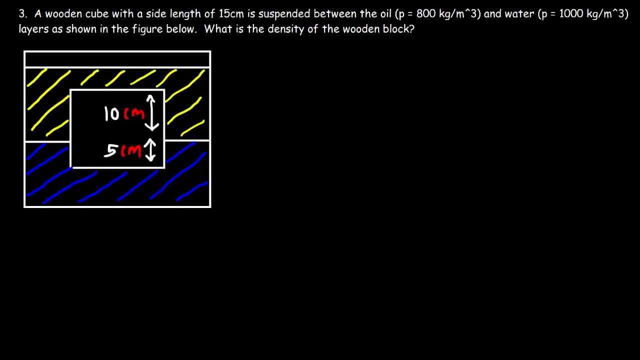 And so it's 9,520 kilograms per cubic meter. Make sure you understand what this equation means. Number 3. A wooden cube with a side length of 15 centimeters is suspended between the oil and water layers as shown in the figure below. 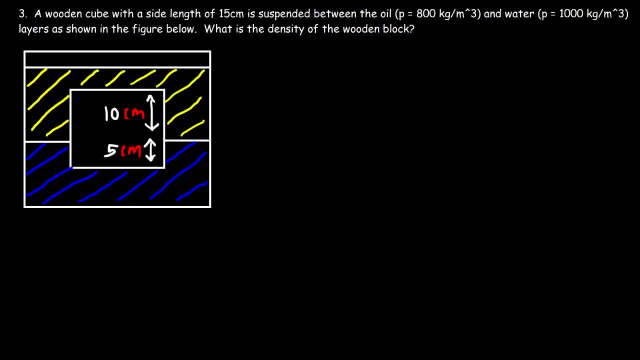 Number 3.. A wooden cube with a side length of 15 centimeters is suspended between the oil and water layers, as shown in the figure below. Number 3. A wooden cube with a side length of 15 centimeters is suspended between the oil and water layers as shown in the figure below. 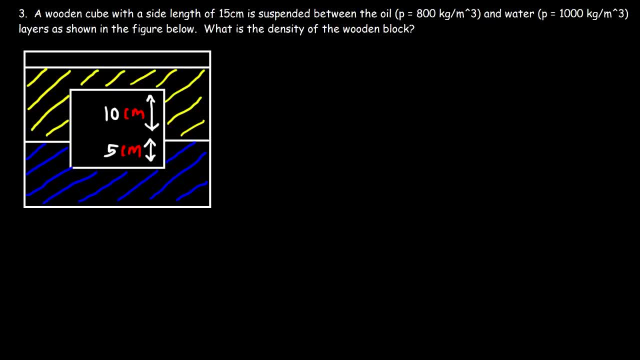 Number 3.. A wooden cube with a side length of 15 centimeters is suspended between the oil and water layers, as shown in the figure below. Number 3. A wooden cube with a side length of 15 centimeters is suspended between the oil and water layers as shown in the figure below. 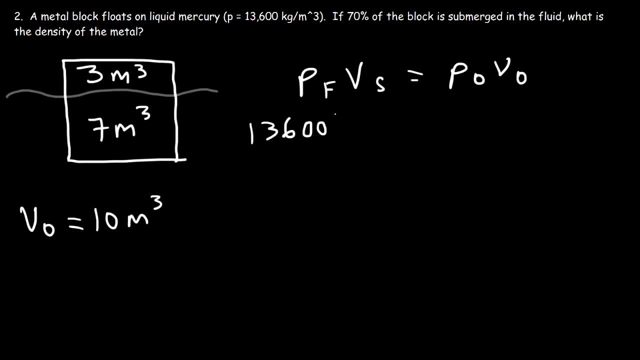 So we have the density of the fluid, That's liquid mercury, That's 13,600.. The volume submerged is 7.. And we're looking for the density of the metal, That is, the metal block And the volume of the entire object. 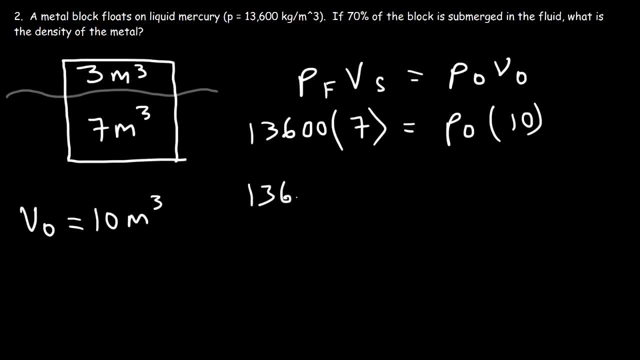 And the volume of the entire object is 10.. So it's going to be 13,600 times 7 over 10.. So if you need to find the density of the object, it's the density of the fluid times, the volume submerged divided by the volume of the object. 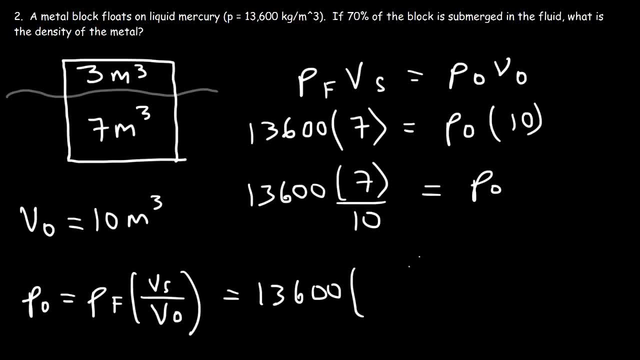 So that's 13,600 times 7 over 10,, which is 0.7 or 70%. So therefore, the density of the metal is simply 70% of the volume of the object. That's the density of the density of mercury. 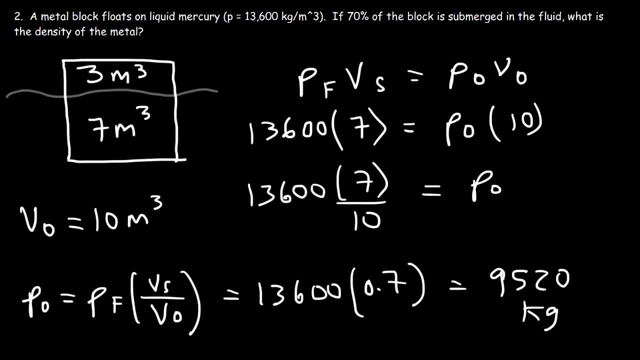 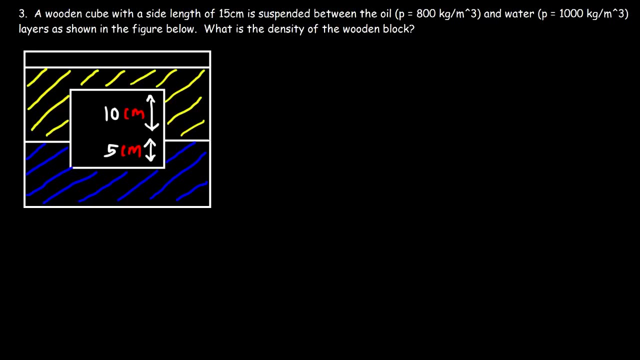 And so it's 9,520 kilograms per cubic meter. Make sure you understand what this equation means. Number three: A wooden cube with a side length of 15 centimeters is suspended between the oil and water layers as shown in the figure below. 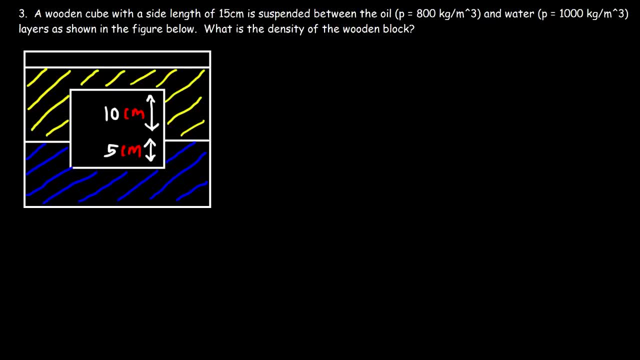 What is the density of the wooden block? Now, if you had to guess, what do you think the density would be? Now the block floats on the water layer, So the density has to be less than 1,000.. We know, light objects float on water. 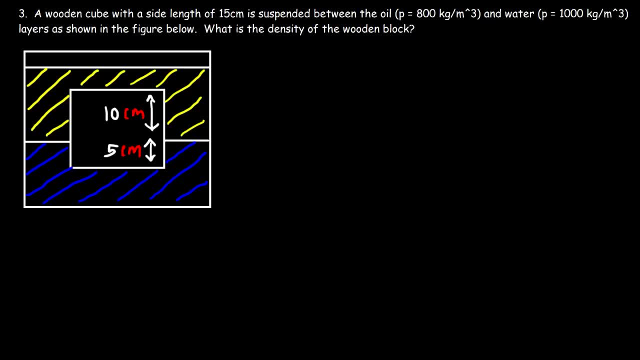 Heavy objects sink. Now the wooden block is not floating on top of the oil layer, It's sinking in the oil layer, So the density has to be greater than 800.. Now, because it stays suspended in between the two layers, the density has to be between somewhere within 800 and 1,000. 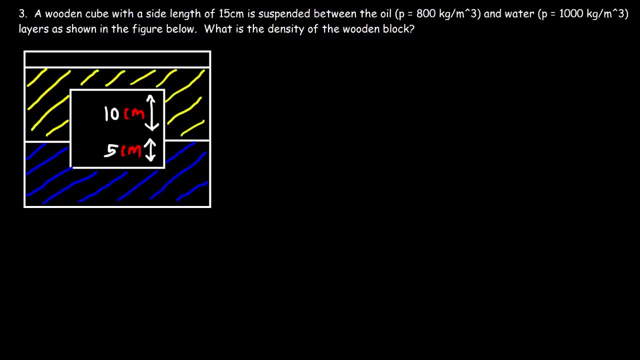 Now here's a question for you: Is the density closer to 800 or is it closer to 1,000?? Is it between 800 and 900 or is it between 900 and 1,000?? Now notice that most of the volume of the block is in the oil layer. 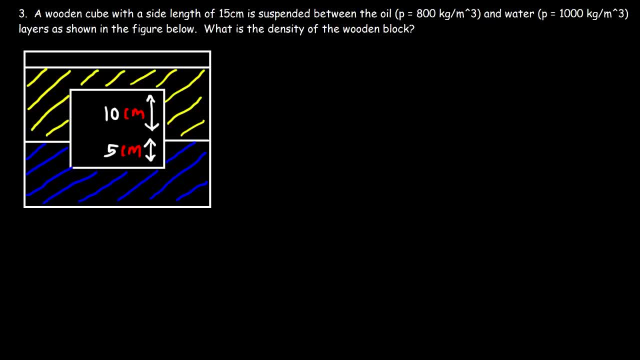 Number 3.. A wooden cube with a side length of 15 centimeters is suspended between the oil and water layers, as shown in the figure below. Number 3. A wooden cube with a side length of 15 centimeters is suspended between the oil and water layers as shown in the figure below. 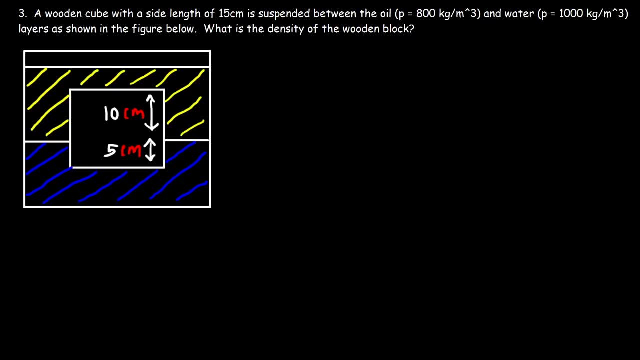 Number 3. A wooden cube with a side length of 15 centimeters is suspended between the oil and water layers, as shown in the figure below. Number 3. has to be less than 1000.. We know light objects float on water, Heavy objects sink. Now the wooden. 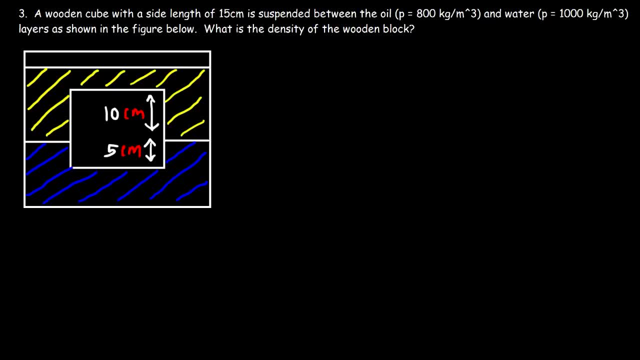 block is not floating on top of the oil layer, It's sinking in the oil layer, so the density has to be greater than 800.. Now, because it stays suspended in between the two layers, the density has to be between somewhere within 800 and 1000.. 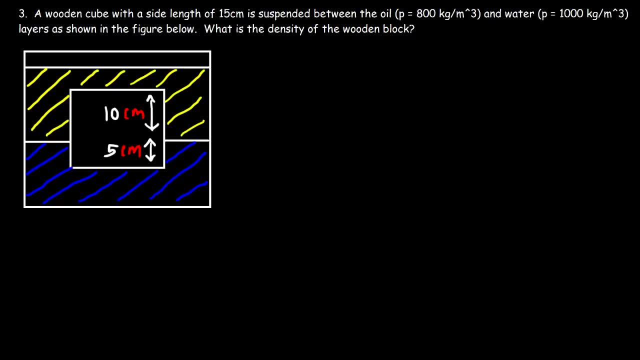 Now here's a question for you: Is the density closer to 800 or is it closer to 1000?? Is it between 800 and 900 or is it between 900 and 1000?? Now notice that most of the volume of the block is in the oil. 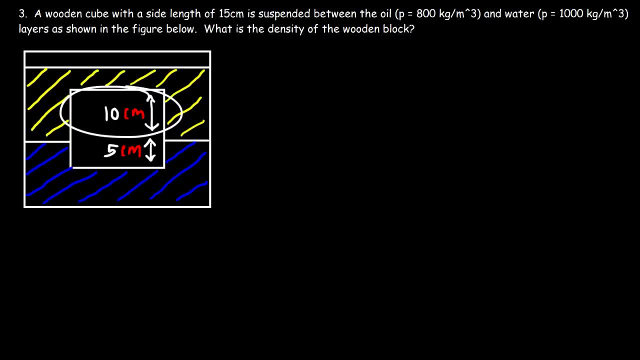 layer. So that means that the density of the block is closer to the density of oil. So we should expect an answer somewhere between 800 and 900.. So how can we do this? In the last problem we were able to calculate the density of the object by 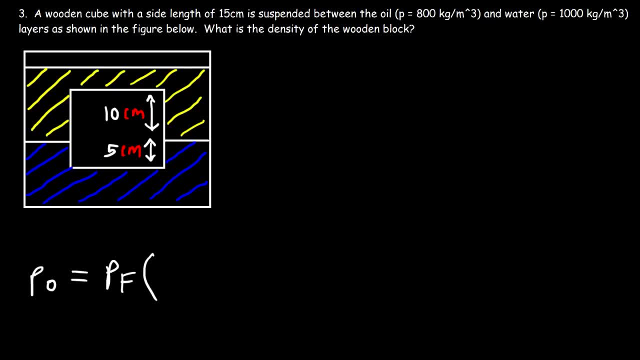 taking the density of the fluid and multiplying by the fraction of the object submerged in that fluid, It was VO over. actually it was VF. I take that back. It was VS over VO. That's the volume submerged divided by the entire volume of the. 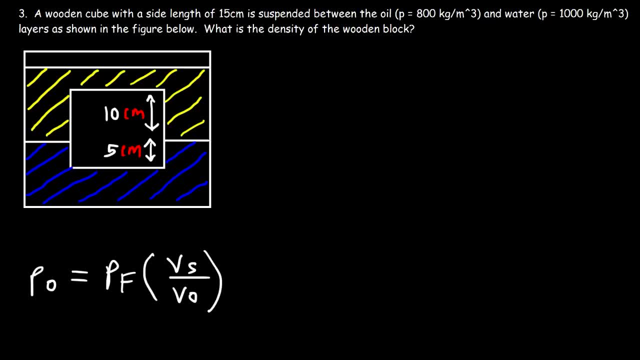 object. Now we're going to use that same relationship, but with two fluids. So the density of the object is going to be the density of, let's say, the water layer, which is, we'll say, rho, one times the volume submerged. 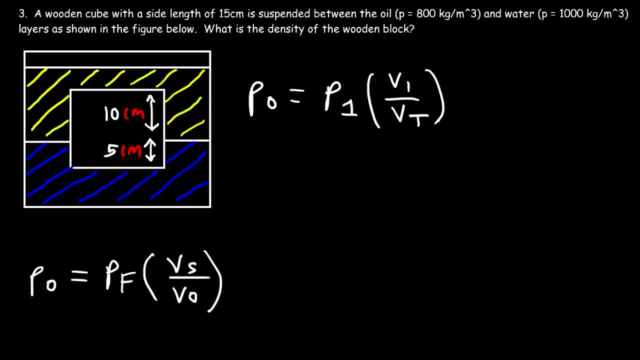 in the water layer divided by the total volume. I'll put VT plus the density of the second fluid times the volume submerged in that fluid divided by the total volume. So that's the easiest way to calculate the density of this wooden block. Now the volume is equal to the area times the height. 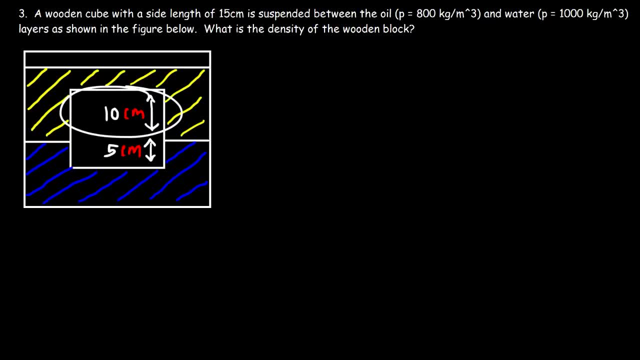 So that means that the density of the block is closer to the density of oil. So we should expect an answer somewhere between 800 and 900.. So how can we do this? In the last problem we were able to calculate the density of the object. 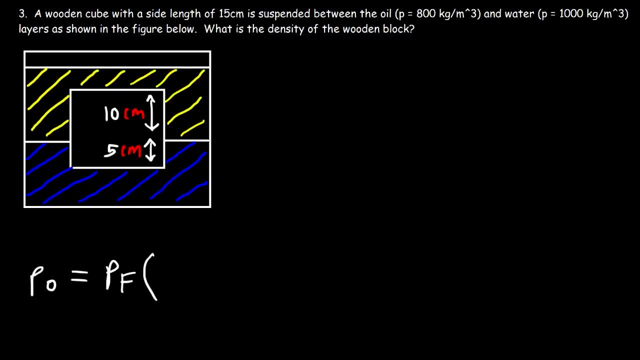 by taking the density of the fluid and multiplying by the fraction of the object submerged in that fluid. It was VO over. actually it was VF. I'll take that back. It was VS over VO. That's the volume submerged divided by the entire volume of the object. 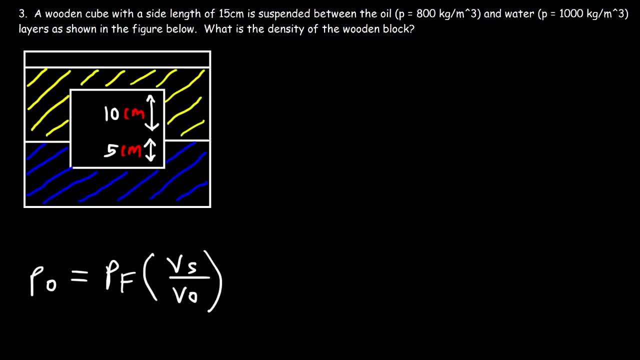 Now we're going to use that same relationship, but with two fluids. So the density of the object is going to be the density of, let's say, the water layer, which is, we'll say, row one times the volume submerged in the water layer divided by the total volume. 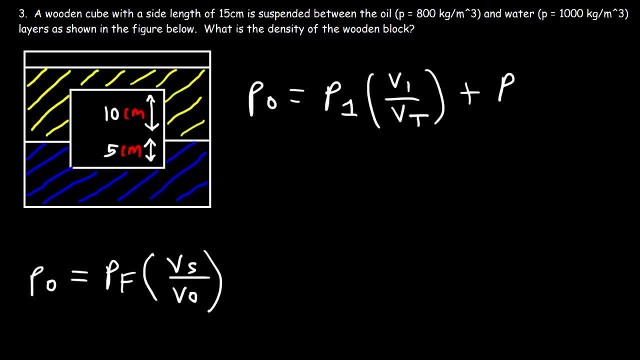 I'll put VT plus the density of the second fluid times the volume submerged in that fluid, divided by the total volume. So that's the easiest way to calculate the density of this wooden block. Now, the volume is equal to the area times the height. 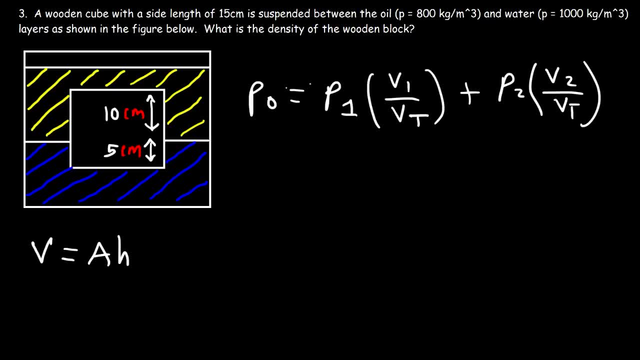 Now, the area is going to be the same. The only thing that's different is the height. The area that's in the water and the oil layer for the cube is going to be the same. It's 15 centimeters by 15 centimeters, but the height is different. 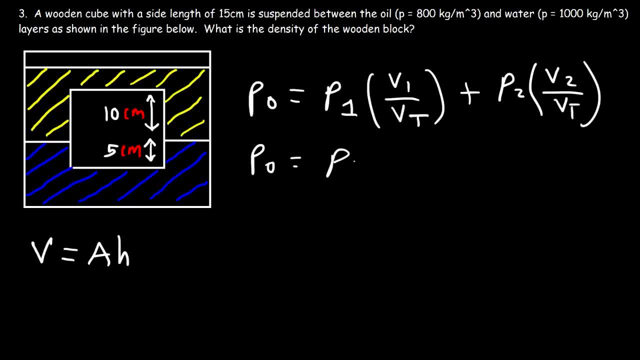 So therefore, we could replace V1 with A times H1.. And the total volume is going to be the area times the total height, which I'm just going to write as H, And then V2 is going to be A times H2.. 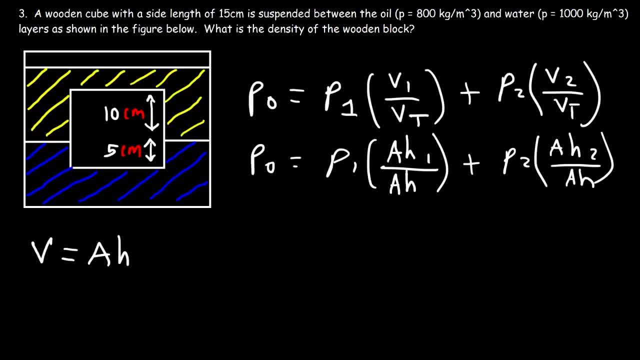 And then VT is A times H once again, So the area portion of the cube will cancel. So that will give us this relationship. The density of the wooden block is going to be the density of the water multiplied by the height of the water, divided by the total height. 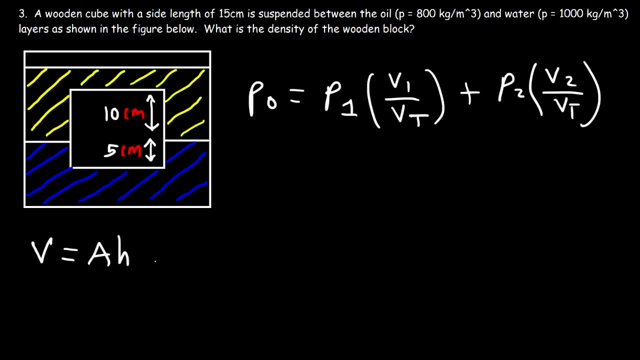 Now the area is going to be the same. The only thing that's different is the height. The area that's in the water and the oil layer for the cube is going to be the same. It's 15 centimeters by 15 centimeters. 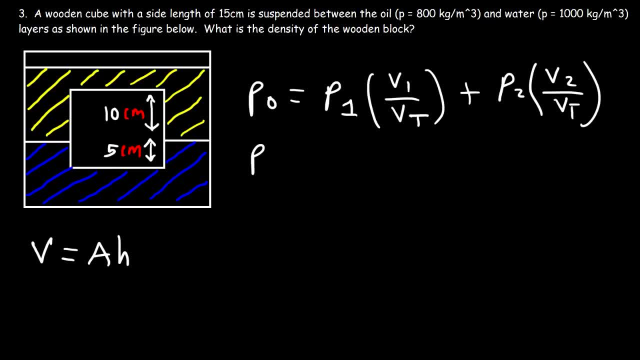 So that's the easiest way to calculate the density of this wooden block. But the height is different, So therefore we could replace V1 with A times H1. And the total volume is going to be the area times the total height. 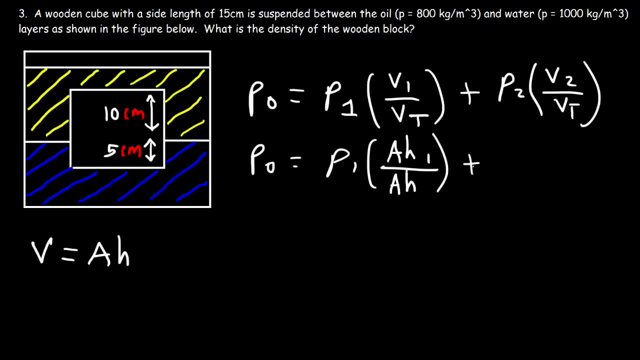 which I'm just going to write as H, And then V2 is going to be A times H2.. And then VT is A times H once again. So the area portion of the cube will cancel. So that will give us this relationship. The density of the wooden block is going to be the density. 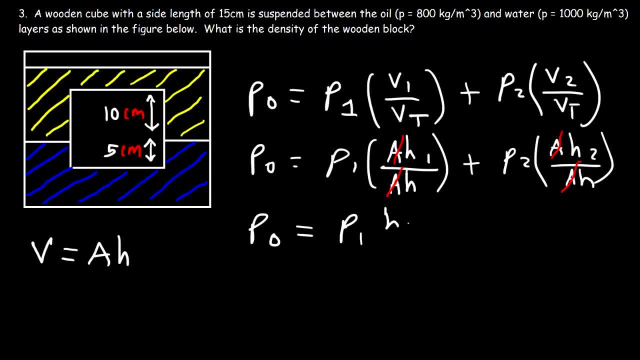 of the water, multiplied by the height of the water, divided by the total height plus the density of the oil, times the height that is submerged in the oil, divided by the total height of the wooden block. So the density of water is 1000 and 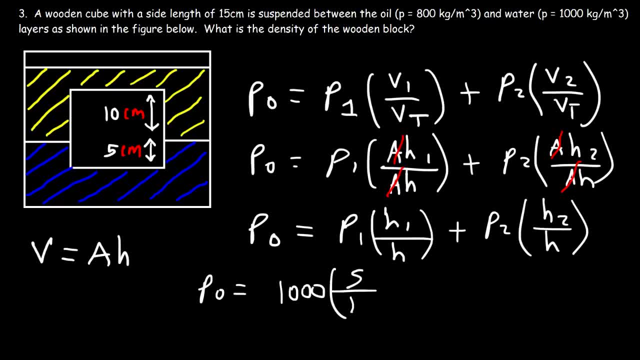 the portion that's at 20 megapiles per volt in this Maintenant that's in water is 5 centimeters divided by a total height of 5 plus 10, which is 15.. And the density of oil is 800. And the height, or the portion that's in the oil later, is 10. 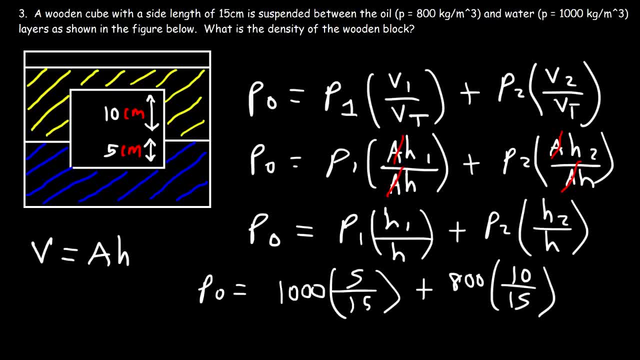 centimeters out of a total of 15.. So, basically, you can calculate the density of the wooden block by taking a weighted average of the density of the oil and the density of the water, And it's based on how much is submerged in the oil and how much is submerged in the water. 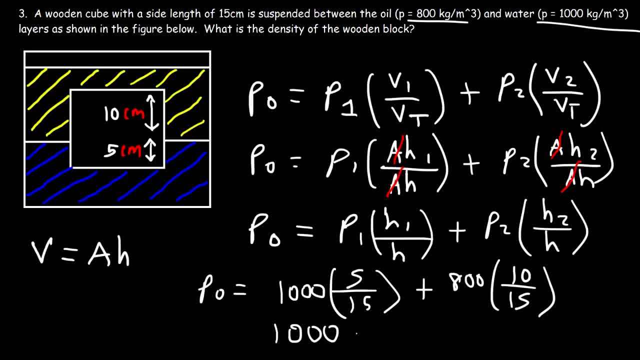 So one-third of the volume of the block is in water and two-thirds is in oil. So that's why the density is going to be closer to 800 than 1,000.. So 100 times a third plus 800 times two-thirds. 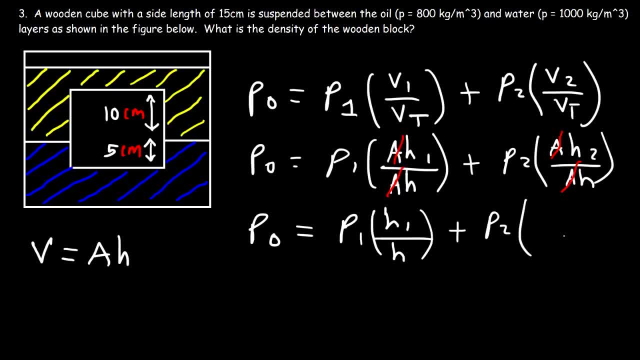 Plus the density of the oil, times the height that is submerged in the oil divided by the total height of the wooden block. So the density of water is 1000. And the portion that's in water is 5 centimeters divided by the total height of 5 plus 10, which is 15.. 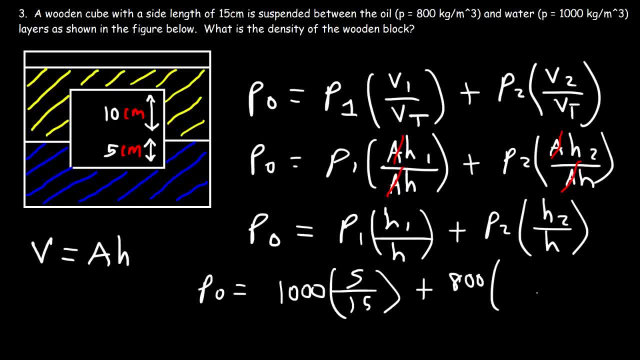 And the density of oil is 800. And the height, or the portion that's in the oil layer, is 10 centimeters out of a total of 15.. So, basically, you can calculate the density of the wooden block by taking a weighted average of the density of the oil and the density of the water. 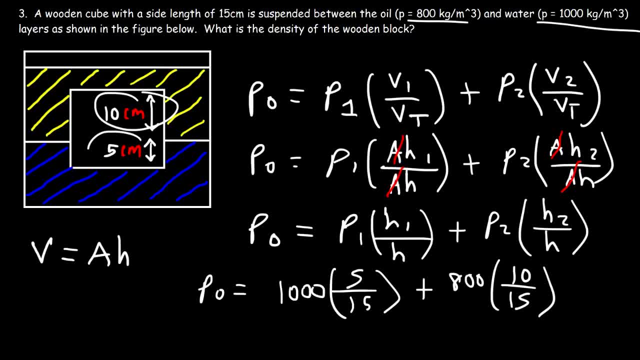 And it's based on how much is submerged in the oil and how much is submerged in the water. So 1 third of the volume of the block is in water And 2 thirds is in oil. So that's why the density is going to be closer to 800 than 1000.. 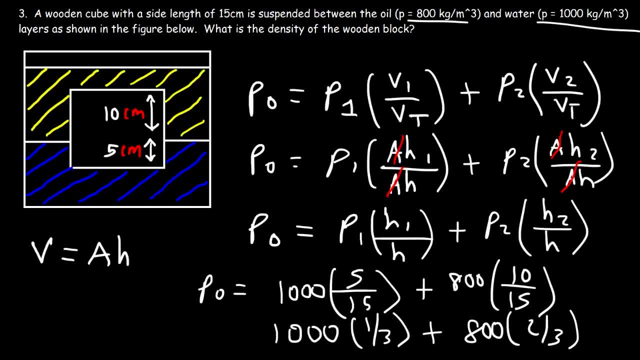 So 100 times 1 third plus 800 times 2 thirds- I meant to say 1000 times 1 third, not 100.. So 1000 times 1 third plus 800 times 2 thirds, That's going to be 866.7 kilograms per cubic meter. 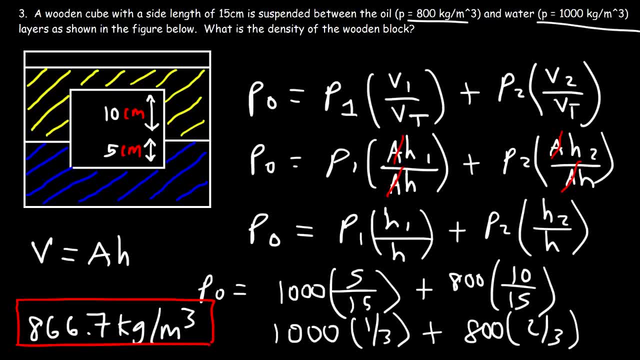 So this is the density of the wooden block. So now let's think about what we have at this moment. So we can see that the density is indeed between 800 and 1000, which is what we should expect, And it's closer to 800 than it is to 1000, since the majority of the block is in the oil layer. 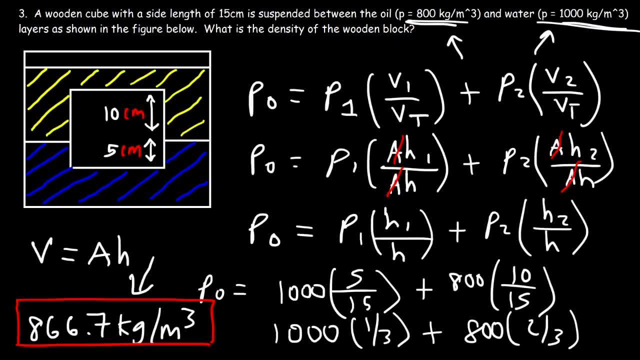 It's between 800 and 900.. Now there's another way in which you can get the same answer. It's a longer way, but if you want to understand it, here's what you can do. If you can calculate the gauge pressure between these two points and also the buoyant force, 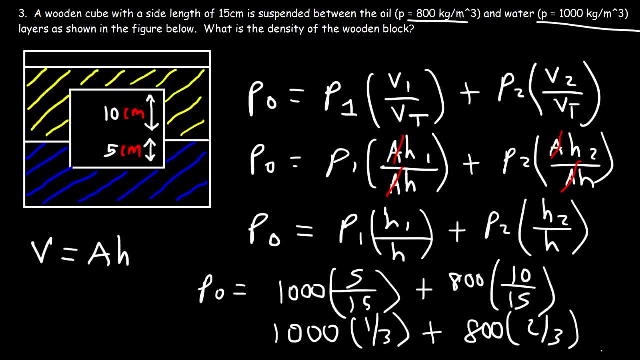 I meant to say 1,000.. 1,000 times a third, not 100.. So 1,000 times one-third plus 800 times two-thirds, That's going to be 866.7 kilograms per cubic meter. So this is the density of the wooden block. 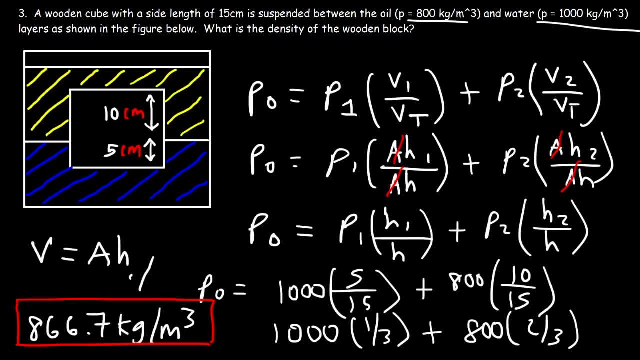 So now let's think about what we have at this moment. So we can see that the density is indeed between 800 and 1,000, which is what we should expect, And it's closer to 800 than it is to 1,000, since the majority of the block is in the oil layer, It's between 800. 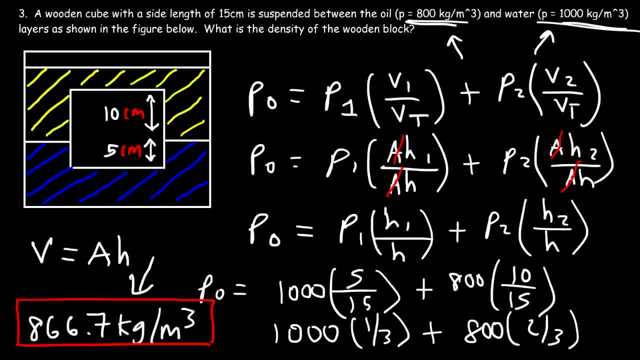 and 900.. Now there's another way in which you can get the same answer. It's a longer way, but if you want to understand it, here's what you could do. If you can calculate the gauge pressure between these two points and also the buoyant force, you can also find the density of the wooden block. You 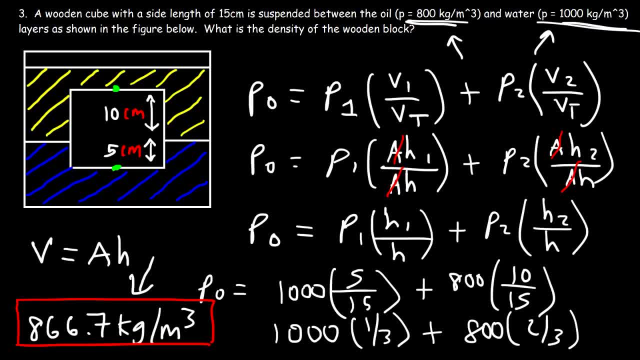 need the mass of the block and the density of the wooden block. So you need the mass of the block and, divided by the volume which you already have, the side length of the cube. So the volume of the cube is just x times x times x. So, using the upward buoyant force and the downward weight force of the 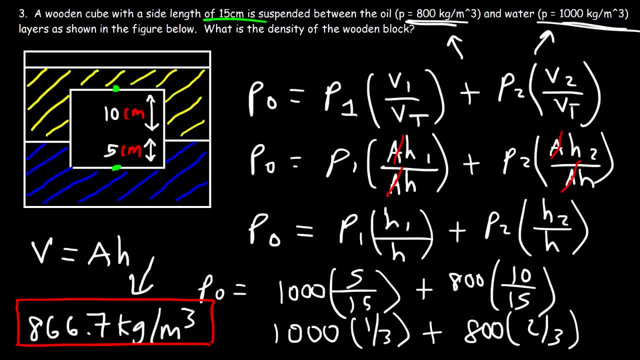 block. you can calculate the mass of the wooden block and thus calculate the density. Now I've shown how to do it, how to solve this exact same problem, getting the same answer, using that other four-hour video on pressure and fluids. You could find it on YouTube or you could find it in my new 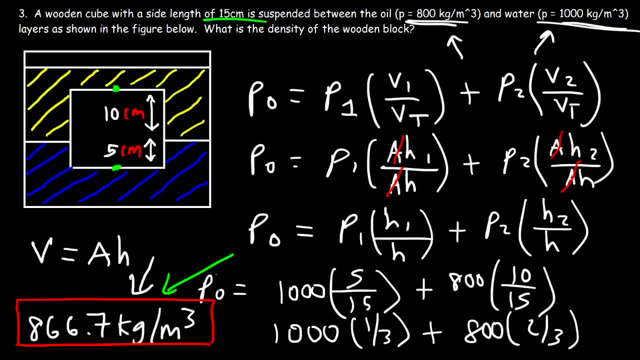 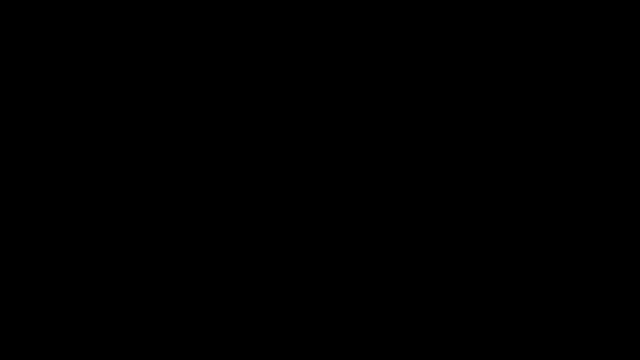 physics video playlist, You should locate it there. But if you want to see that other way in which to calculate the density of this block, the same exact problem- feel free to check out that video. Subtitles by the Amaraorg community. 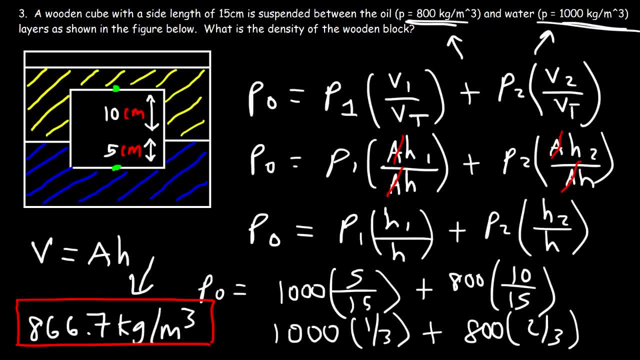 you can also find the density of the wooden block. You need the mass of the block and divide it by the volume which you already have: the side length of the cube. So the volume of the cube is just x times x times x. So, using the upward buoyant force and the downward weight force of the block, 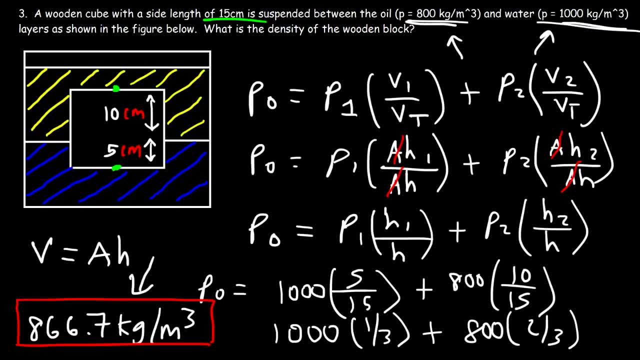 you can calculate the mass of the wooden block and thus calculate the density. Now I've shown how to do it, how to solve this exact same problem, getting the same answer using that other technique, And it's in another, like 4-hour video on pressure and fluids. 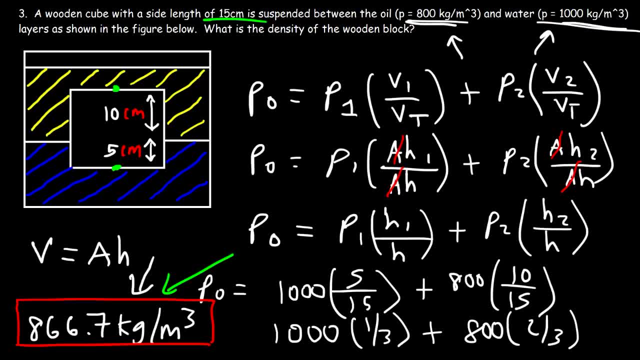 You can find it on YouTube or you can find it in my new physics video playlist. You should locate it there. But if you want to see that other way in which to calculate the density of this block, the same exact problem, feel free to check out that video. Thank you. 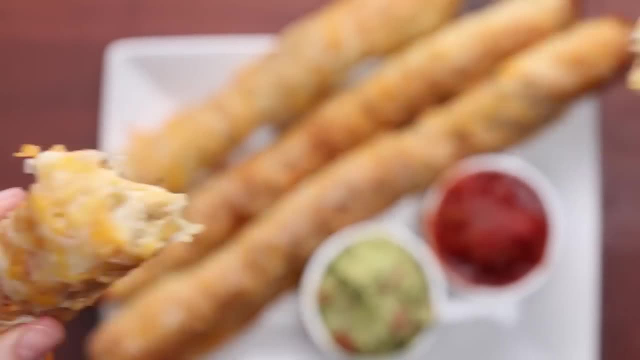 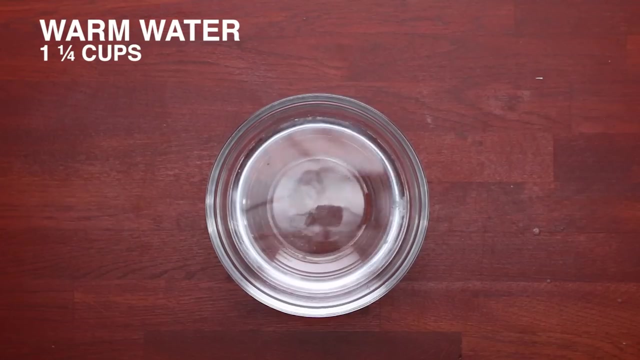 Hey there, I'm Claire. I'm a Tasty producer and today I'm going to show you some of my favorite recipes to make for the kids in my life. Personally, I don't actually have kids, but my mom and I are the caregivers for my six-year-old. 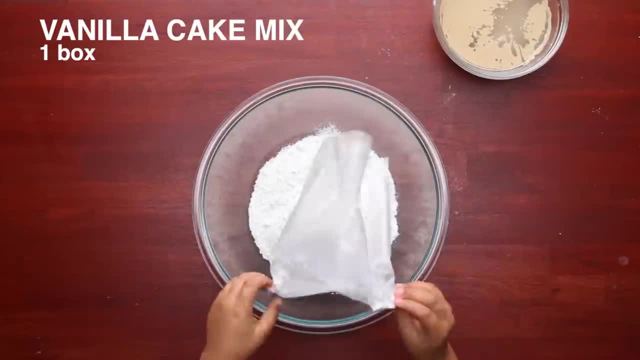 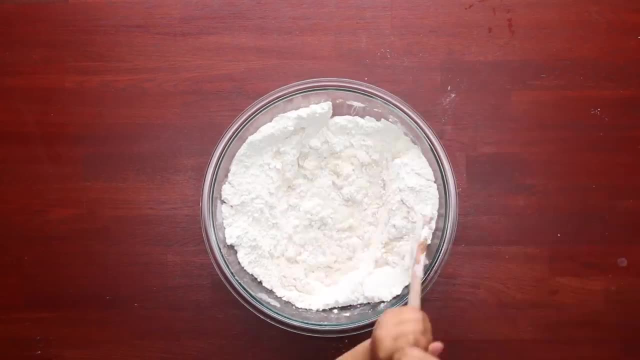 niece and my three-year-old nephew. Basically, I get to be this really cool anti-mom hybrid superhero and it's hard, but it's also really, really rewarding. When they suddenly came into my care, I had to quickly learn how to cook for kids and let me tell you it was. 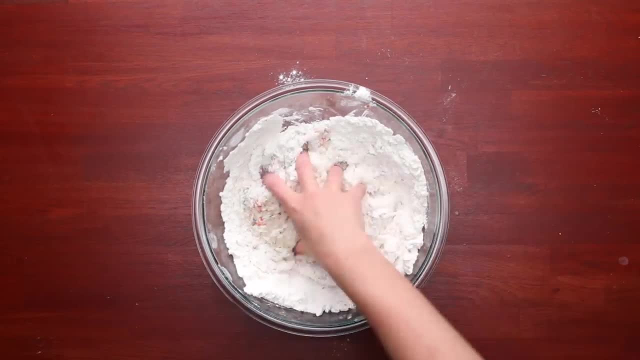 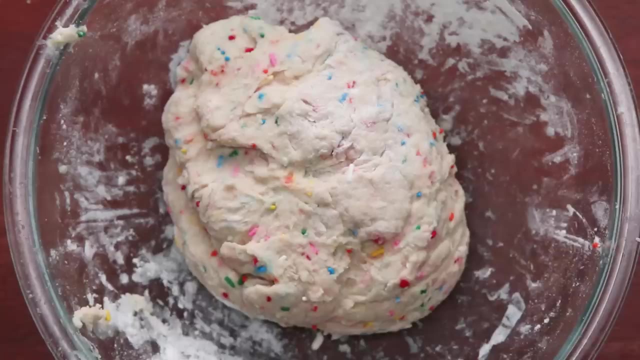 no easy feat and I was lucky enough to be able to channel it into my work by making Tasty videos and Tasty Junior videos. My coworker Hannah. she has this six-year-old son. His name is Jackson and he's my best friend and he's usually my sous chef in all Tasty. 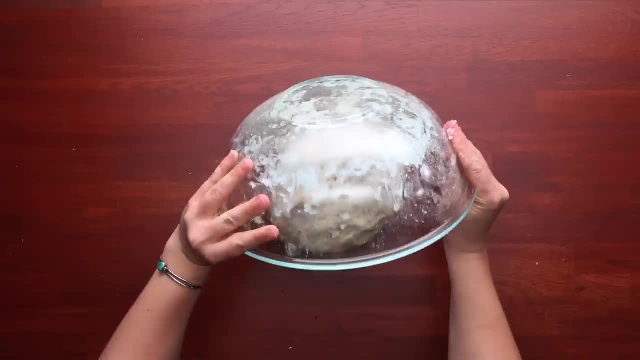 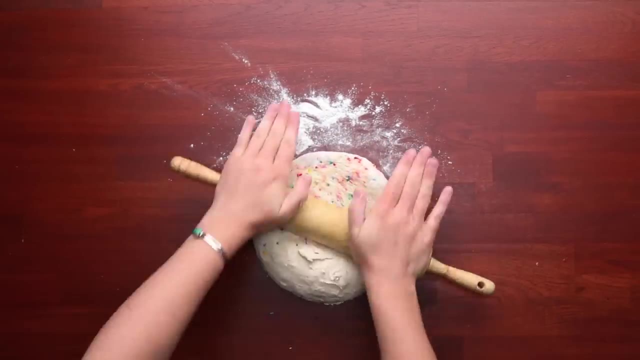 Junior videos. We have been cooking together since he was four and I've gotten to see him blossom into such a kind-hearted and goofy boy. We have a blast together in the kitchen and he brings so much joy to the office whenever he comes in. So, as all parents know, you.